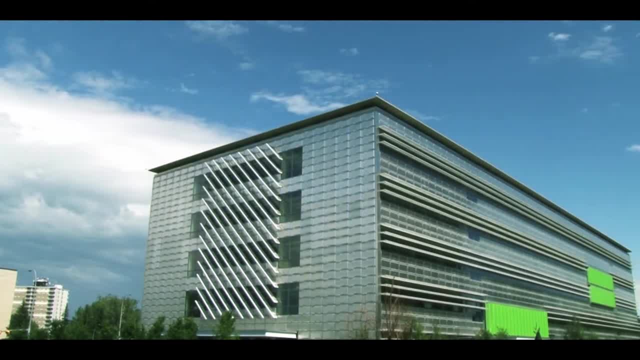 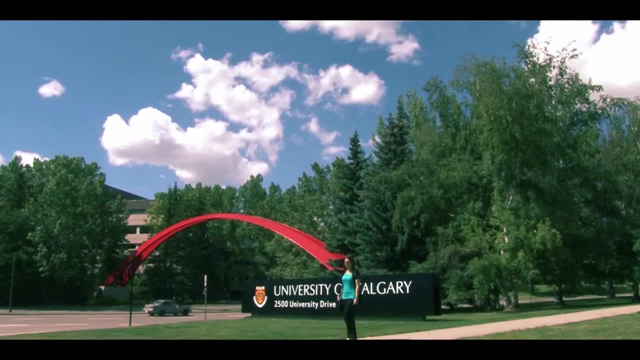 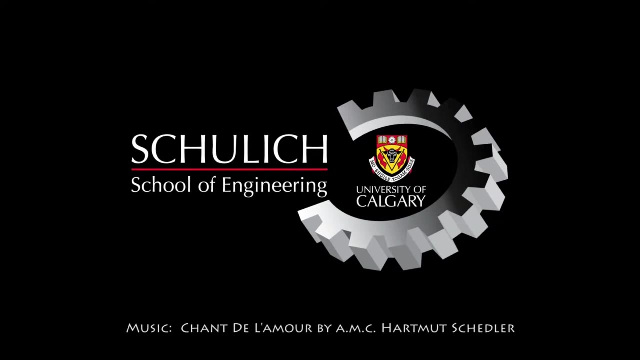 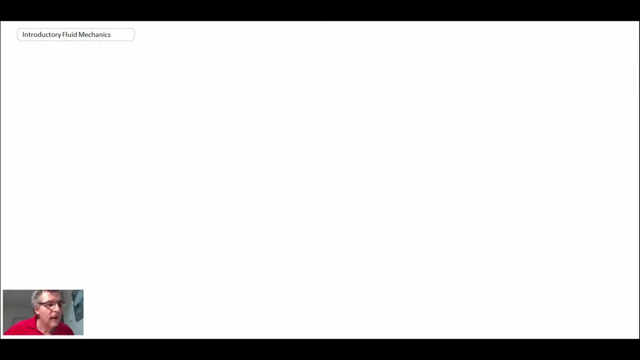 In the last segment. what we did is we took the governing equations and we performed Reynolds averaging to them and we came up with expressions and came across the turbulent stresses, and these are things that make it difficult for us to solve for the velocity profile mean. 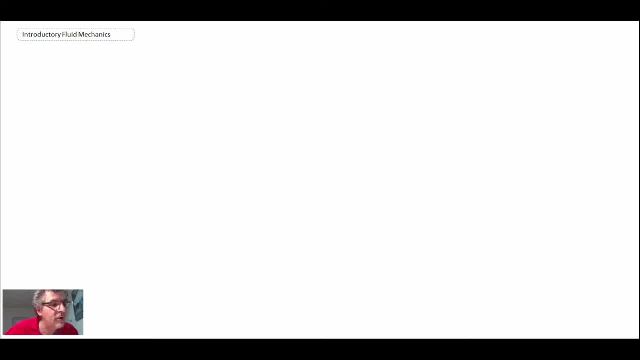 velocity profile and turbulent flow fields, But it turns out that we can make orders of magnitude estimates here and we can eliminate some terms, and so that's what we're going to look at now, and we're going to come up with velocity profiles that enable us then 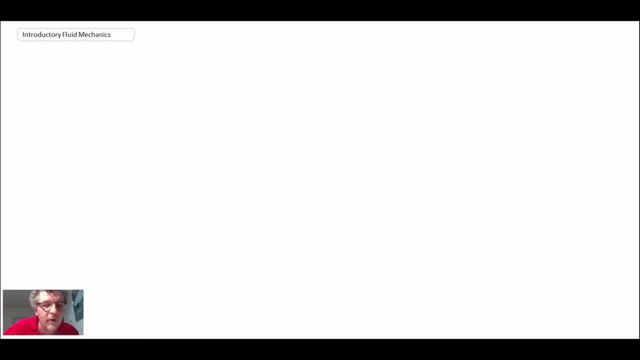 to move in the direction of getting the friction factor for turbulent pipe flow. So it turns out that if we're looking at duct flow, such as pipe flow or boundary layer flow, the minus rho u, prime, v, prime term is the most dominant turbulent stress and 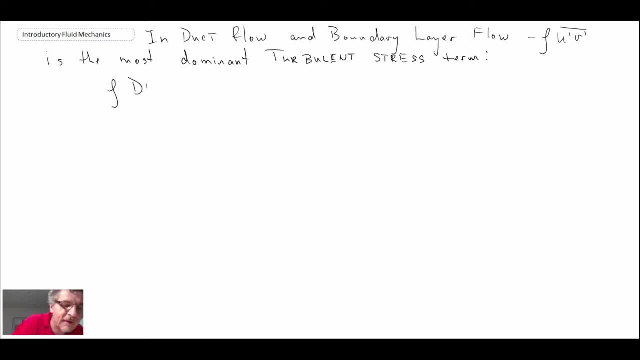 consequently, the governing equation, specifically the Navier-Stokes equation, can be written in the following manner: as an approximation- And what I've done here is I've left the last term- in terms of a shear stress, and the reason for that is when we're dealing with turbulent flow, such as duct flow or 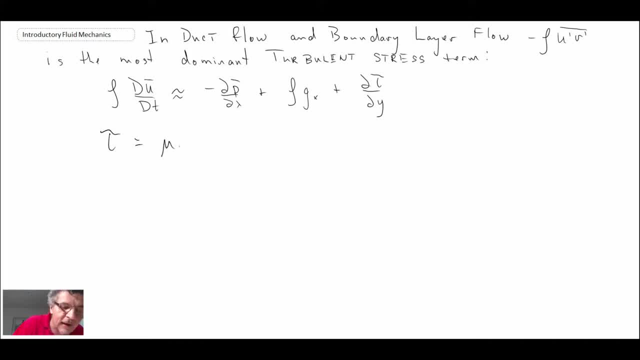 boundary layer flow, we'll approximate the shear stress as being a combination of a laminar contribution and a turbulent stress contribution, And so we have a shear stress of a laminar contribution and a turbulent stress contribution. So we have tau laminar plus tau turbulent. 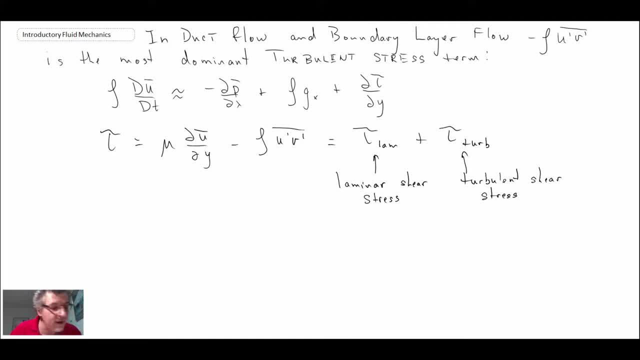 So a lot of this work took place back in the 1920s- 1930s, and what the researchers found was that the laminar shear is mainly right near the wall, And for that reason they often refer to this as being the wall layer or wall region. 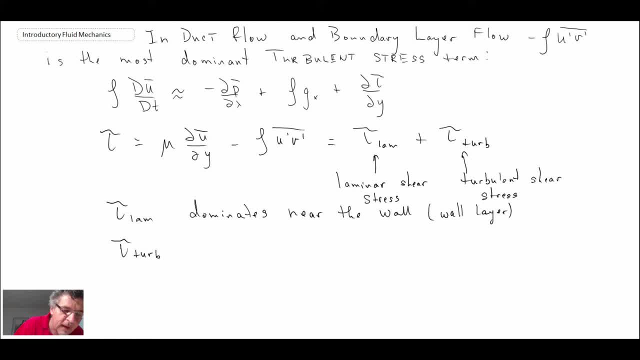 And tau turbulent that dominates further out and that is referred to as being the outer region or outer layer. And so if you look at the velocity profile with a turbulent velocity profile and you look at the shear stress, you can see that the turbulent velocity profile is the outer. 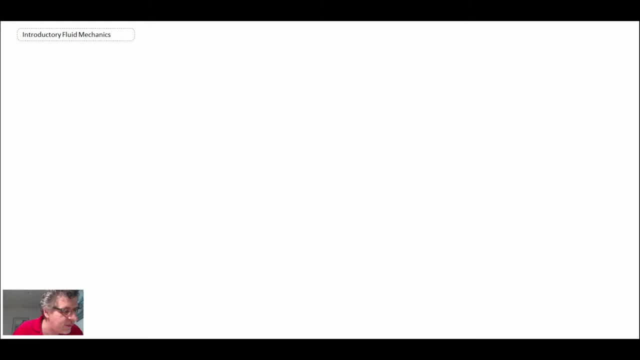 layer, And if you look at the shear stress, you can break it into a laminar and a turbulent component, And so that's what the researchers did years and years ago, And so what we're going to do, let's draw that out. 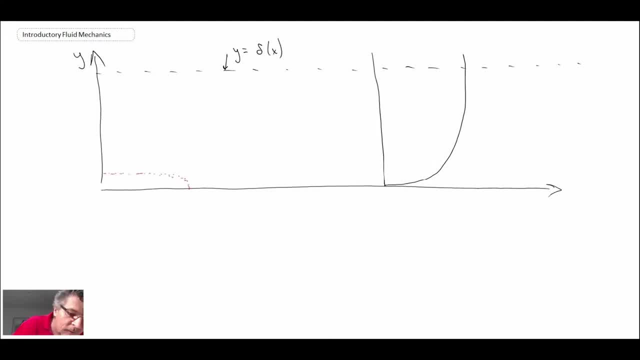 And so what we're going to do, let's draw that out. And so what we're going to do, let's draw that out. So if we were to look at the turbulent stresses in the velocity profile for either pipe flow or a flat plate boundary layer, what we find is that there's the viscous wall layer and 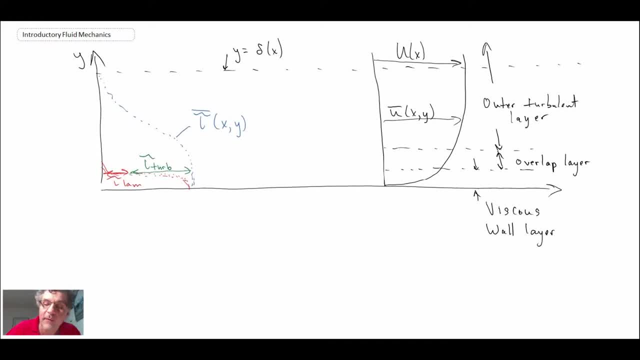 that's where the viscous shear dominates. Then we move into an overlap region, which is in here, and that's where you both have turbulent stress as well as viscous stress being important. And then you get into the outer turbulent layer, where the layer where the turbulent 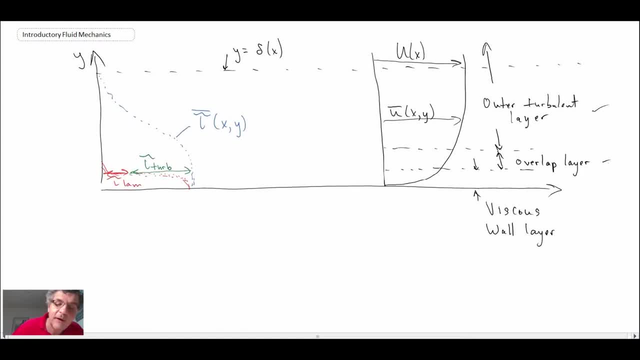 shear stress is the thing that dominates. So if we were to write this out, we have wall layer, We have the outer layer and that would be where the turbulent shear stress is. So if we were to write this out, we have wall layer and that would be where the turbulent 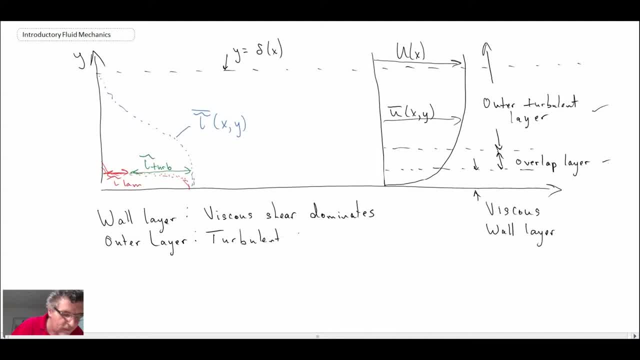 shear dominates. And then we have the overlap region or overlap layer, and that's where both of them are important. So both laminar and turbulent shear is important. So what we're going to do is we're going to proceed forward, and I'll show you three. 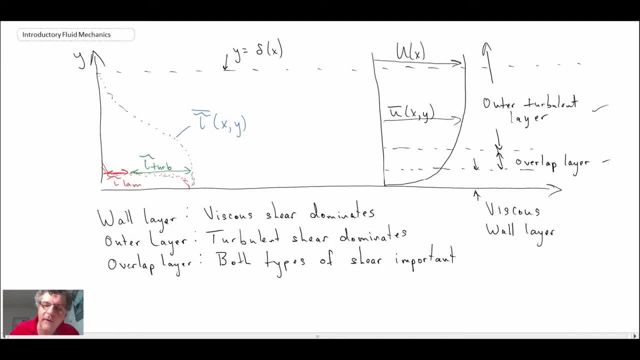 different velocity profiles that were developed back in the 1930s by Millikan von Karman and Prandtl. And in order to do this, we're going to drop the bar from Ubar Ubar, Ubar Ubar. 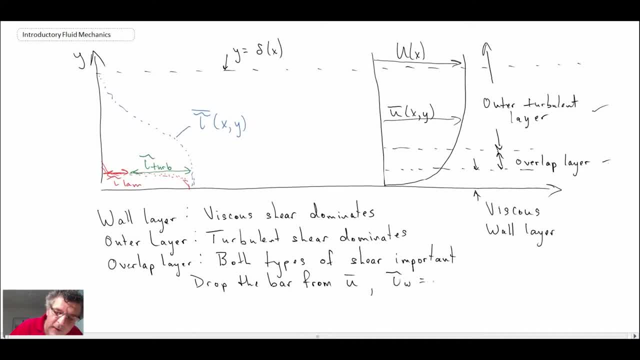 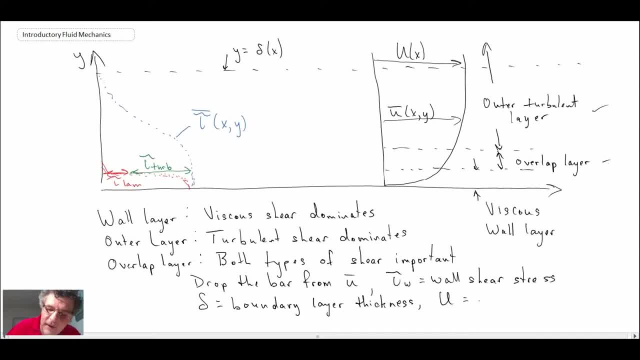 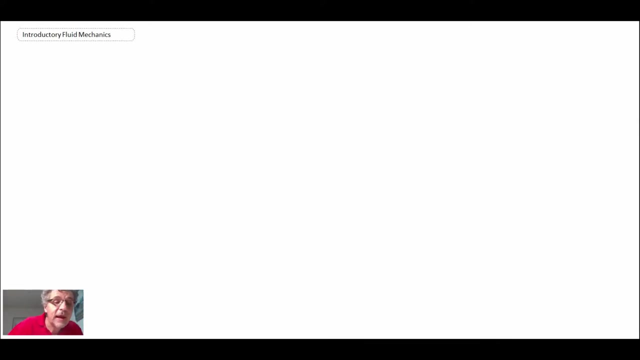 And capital U is velocity at edge of the boundary layer. Okay, So we're going to use those things, And what Prandtl and von Karman and Millikan did is they went through and they came up with velocity profiles. A lot of this was using dimensional analysis as well as experimentation. 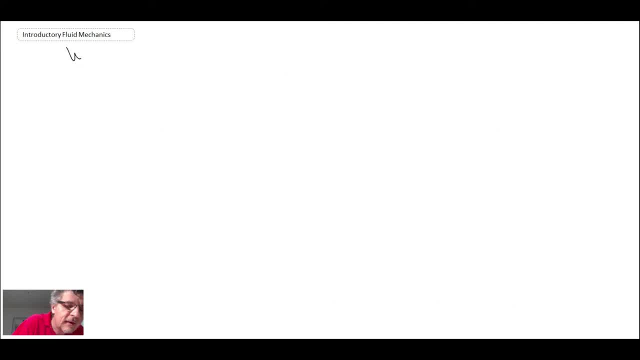 as well as experimentation, but velocity profile for the wall layer was developed by Prandtl Ludwig Prandtl- he was at Göttingen when he did this, and this was in 1930, and he came up with an argument saying that the velocity in the layer 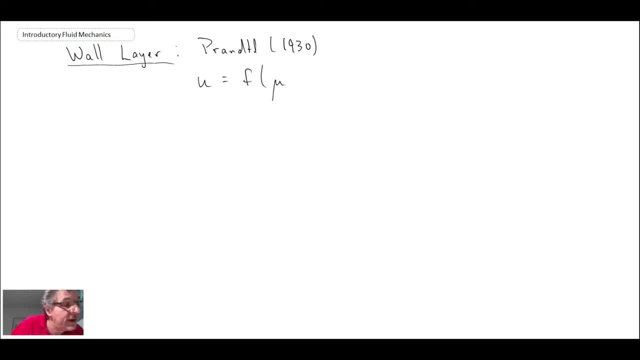 was a function of the viscosity which it would be in the wall layer, the wall shear, stress, the density of the fluid and the distance away from the wall, and using dimensional analysis he was able to come up with a thing called the law of the wall. and he used transform coordinates, so he took the velocity and 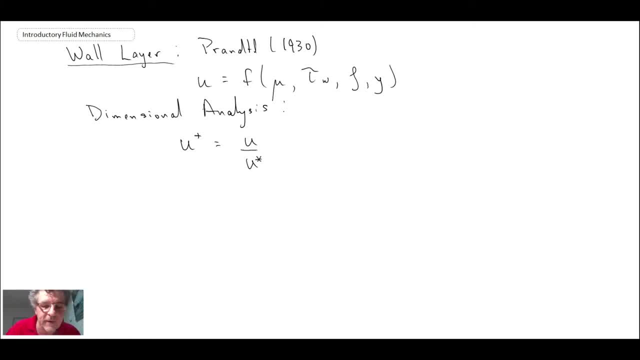 he divided by this u star which is called the friction velocity, which I'll define in a moment, and he found that that was equal to a function of Y, the friction velocity again, and then the kinematic viscosity, and this term here he denoted as Y plus. so we gave that a transform coordinate, and 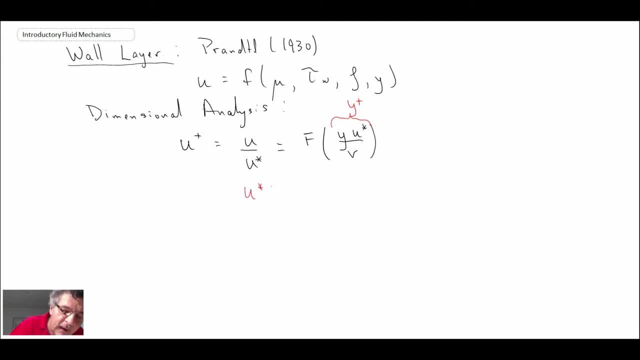 then u star was equal to tau wall. so the shear stress divided by density to the 1 half, and this is the friction velocity. And so this here is equation 1, and it's also known as law of the wall. And so that was Ludwig Prandtl, 1930. 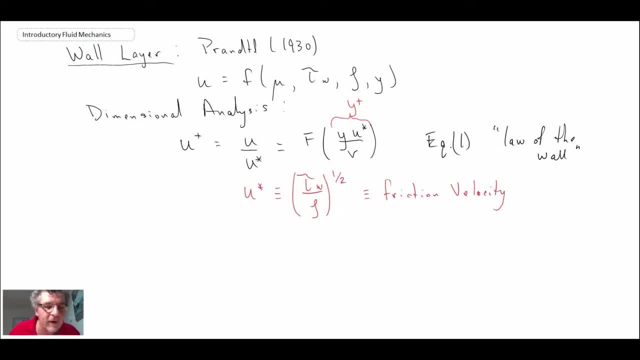 His student was Theodor von Kármán and they were competing with one another quite often in terms of deriving these equations, and they von Kármán. he was probably at Aachen when he developed this, So it was after he left, being a student of Ludwig Prandtl. 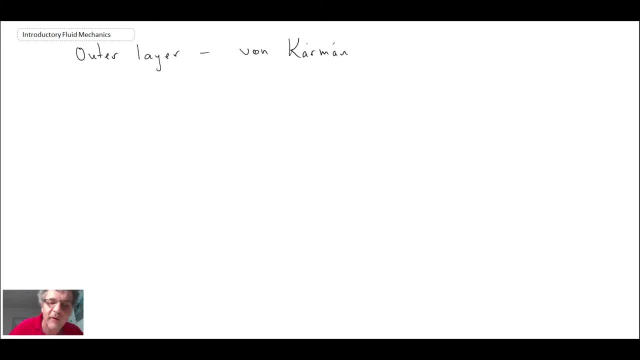 And von Kármán, incidentally- eventually came to the US and started the, the Guggenheim Aeronautical Laboratory at Caltech, where he was very instrumental in the starting of it. But he came up with the velocity profile for the outer layer. 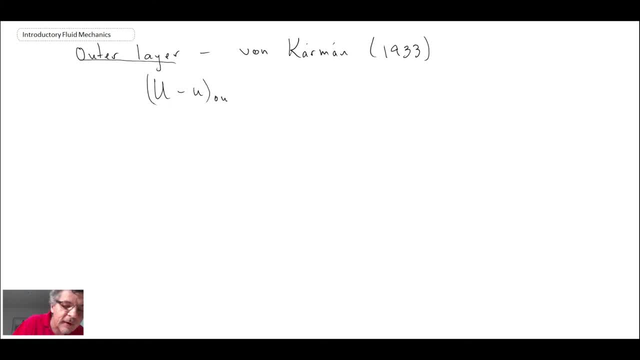 So this is where turbulence shear is important. And again, dimensional analysis. that's really all that they had at their disposal other than that and experimental data, which at the time, was not the greatest. They accomplished great things with what they had. So dimensional analysis. 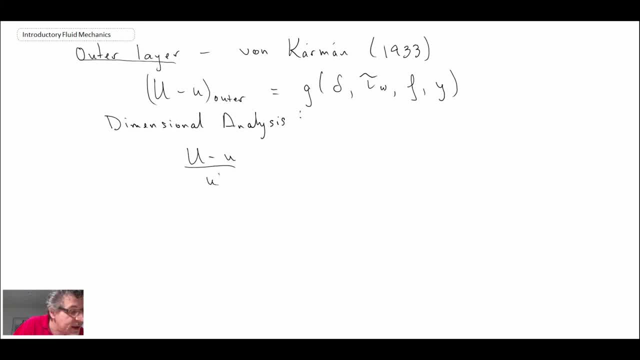 And von Kármán was able to come up with this relationship, And he did scaling based on the boundary layer thickness, that's delta there. This is equation two, And this is referred to as being the velocity defect law. So we have law of the wall. 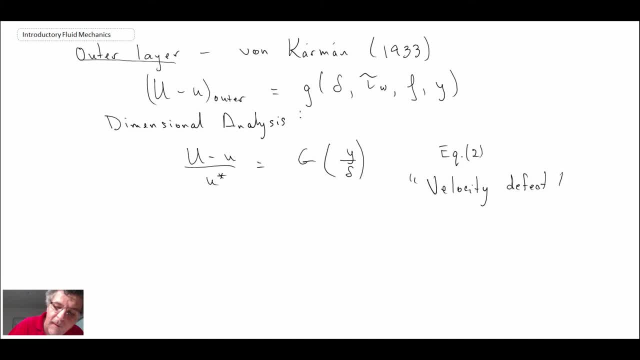 We have velocity defect law And that was in the outer region or the outer layer, And then in the middle, the overlap region. This was investigated by a fellow named Millikan And he looked at pipe flow as well as channel flow And in about 1937, he came up with a velocity profile, again using Ludwig Prandtl's friction velocity and y prime coordinate. 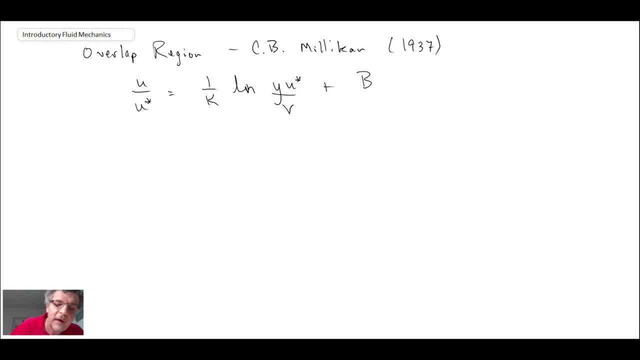 So he came up with this relationship and here k is equal to 0.41, and b, he said, was 5.0, and that was based on the experimental data that he had. These numbers are constantly being fine-tuned as people get more and more data for boundary layers, turbulent boundary layers. 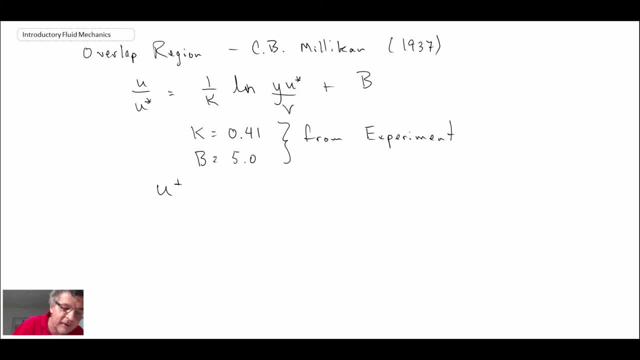 But in here he also defined. He defined a u plus, which was velocity divided by the friction velocity, and he had a y plus, which was y times the friction velocity divided by nu. Remember, the friction velocity was our shear stress at the wall divided by density, square root of that. 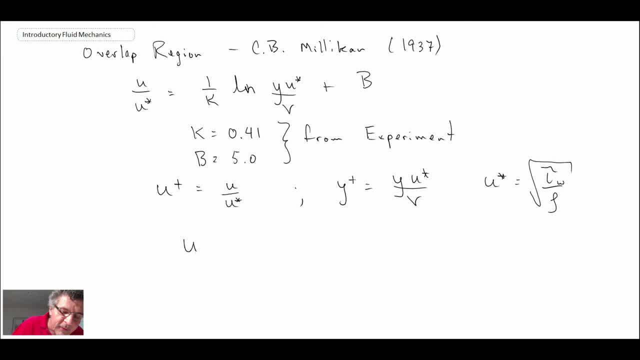 And consequently, what Millikan was able to come up with was this expression, And this we will call equation three. Now, it turns out that this is the equation that applies for quite a bit of the boundary layer, and it's quite representative of the velocity profile for a turbulent boundary layer. 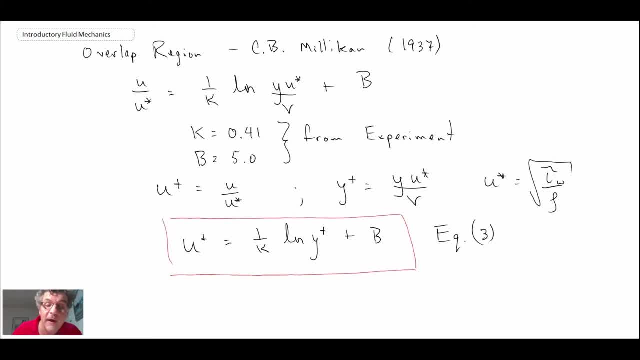 And consequently, that is what we are going to use as we move into the next segment, where we will look at developing a relationship for the friction factor for turbulent flow. It is quite remarkable when you look at all the things that von Karman, Millikan and Prandtl were able to do. 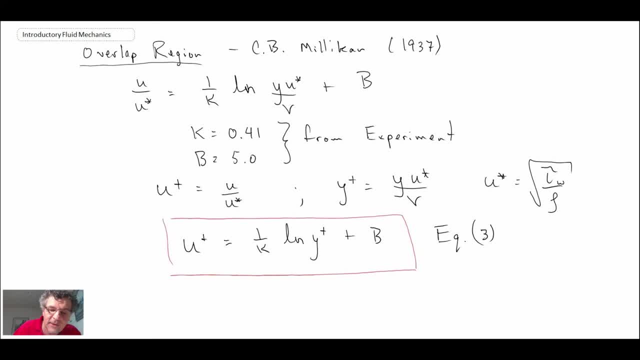 This was all based on dimensional reasoning, dimensional analysis and experimentation. But give them credit. They did not have the fancy tools that we have nowadays with time-resolved particle image velocimetry, laser Doppler velocimetry, Even hot wire anemometry. and if they did, it was very, very primitive electronics that were involved in those systems. 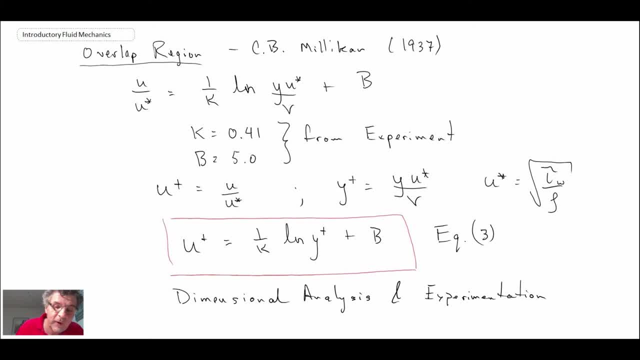 So those are the regions. we are going to use this one as we move into coming up with a relationship for the friction factor, which we will do in the next segment.